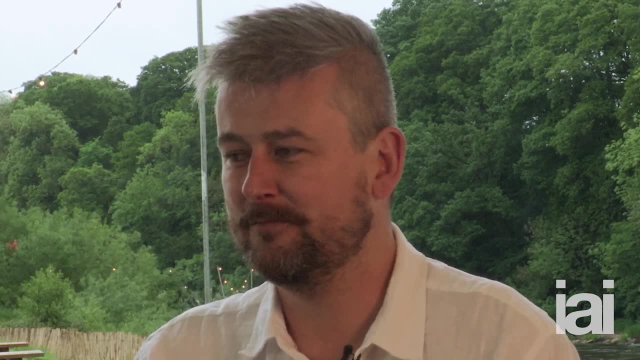 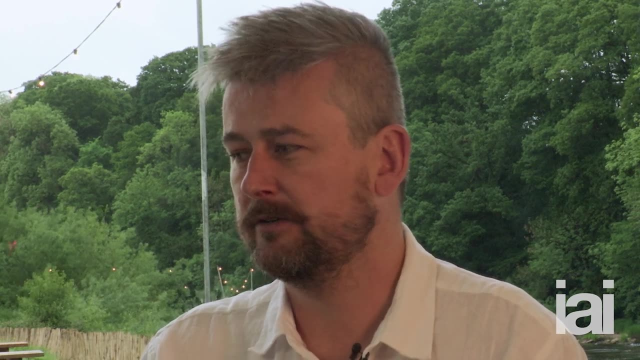 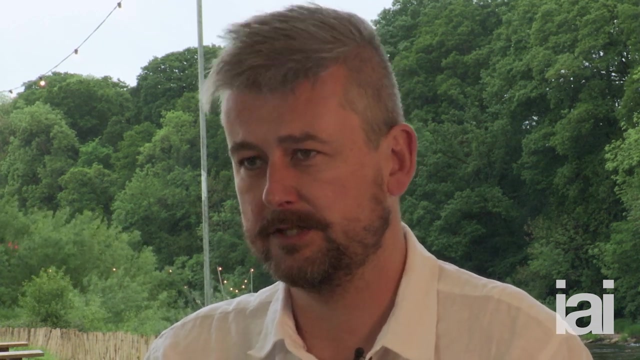 so I had to rethink last year. Now I'm working in a different mode. I'm looking at the data and looking for glitches. So we predict with the standard model of particle physics- That's the current knowledge that we have. We predict how the data should look from the collisions between two protons at 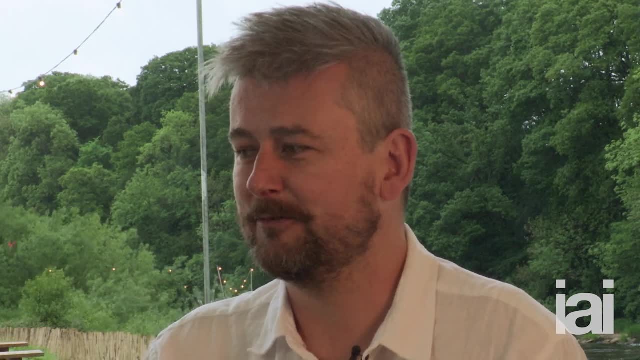 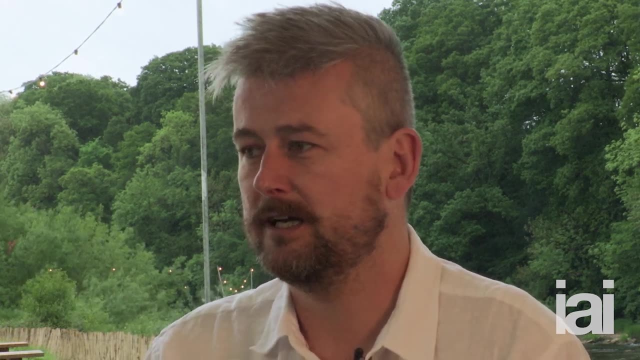 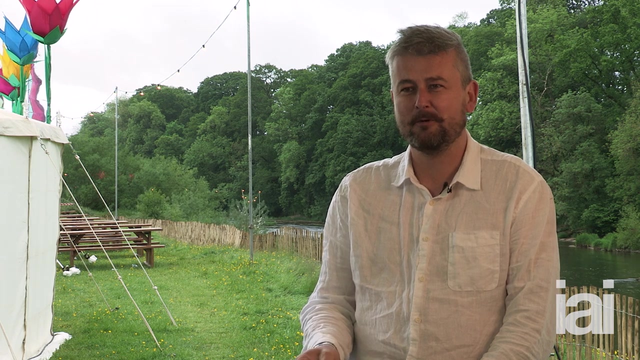 CERN at high energies, And we look for cases where the model disagrees, the prediction disagrees with what's seen, And then that for me is an opportunity. So then we jump on that and try and explain it. but explain it in a very simple way. We kind of just bung in an extra force or an 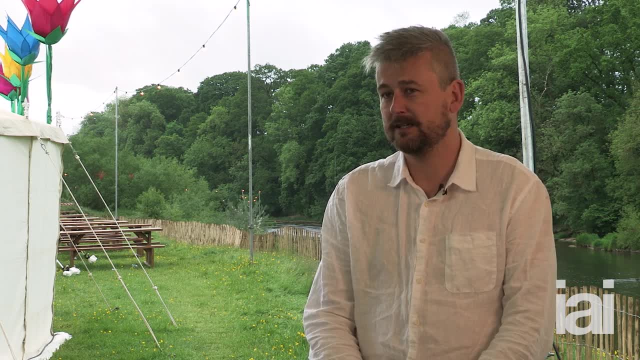 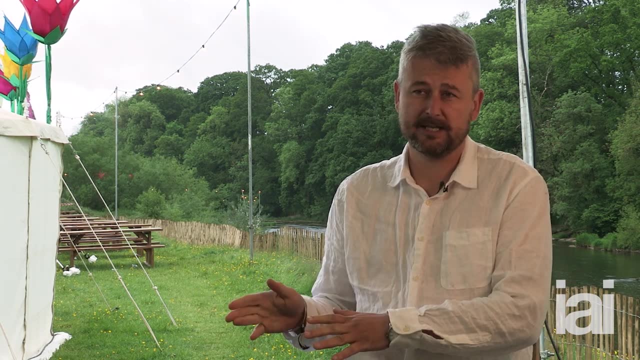 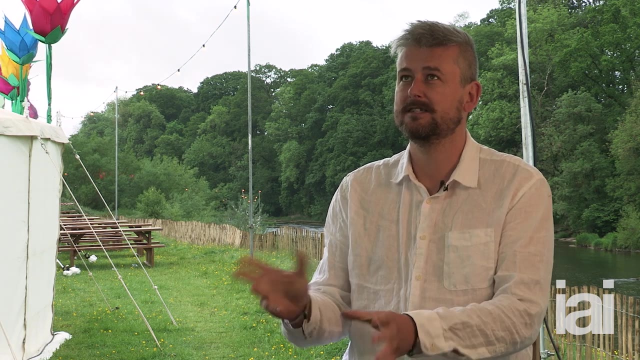 extra particle that would explain what's seen, And then we do some proper phenomenology So we try and suggest other ways in which it may be tested. We first of all check that it's consistent with all other data and then suggest other ways you can sieve the data. 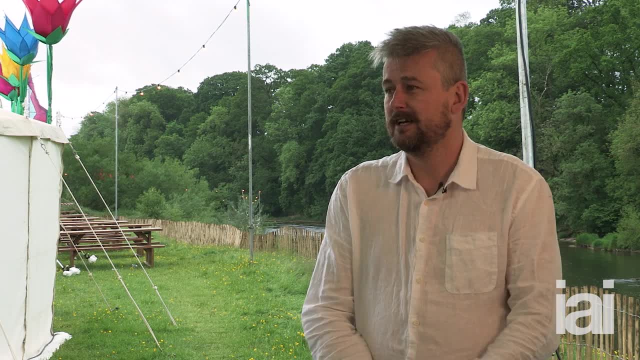 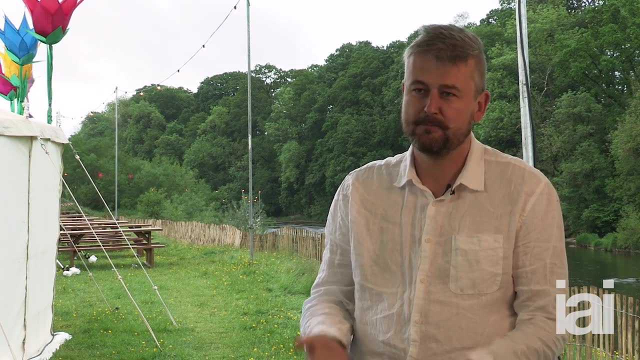 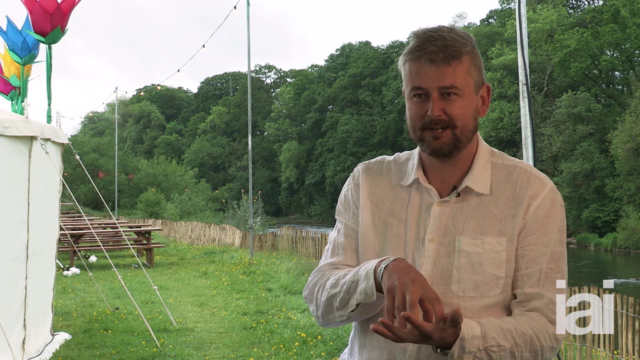 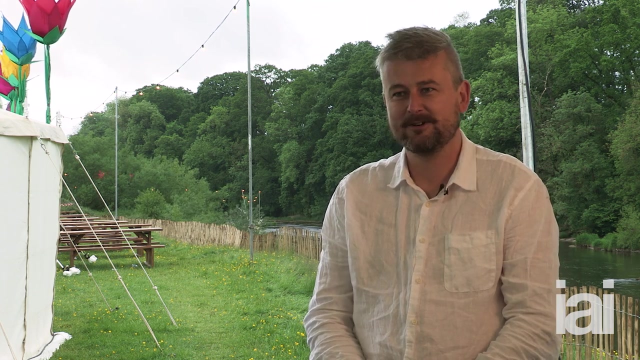 to look for these things And then we go one step further in the theoretical direction. So this is more we call it bottom up science, working from the data and where you've got really solid foundation and you think you know what's going on, And then making hypotheses away from that. So I'm enjoying. 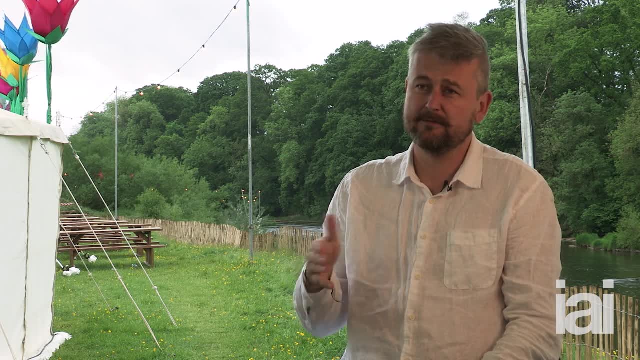 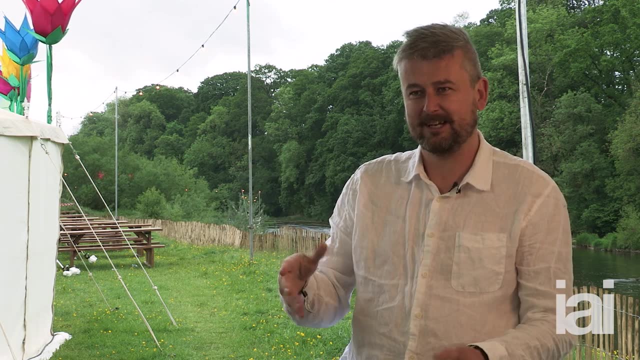 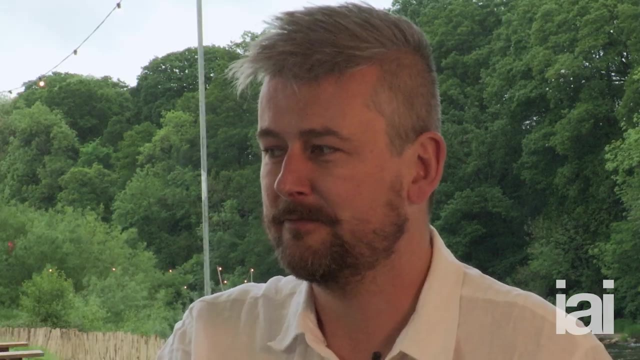 this new way of working. It's certainly quite different to the previous way, where you try and solve everything And make loads of assumptions. That's what we call top down. It's like you start from pure thought and then try and get to experimental observations. But for me, anyway, that approach 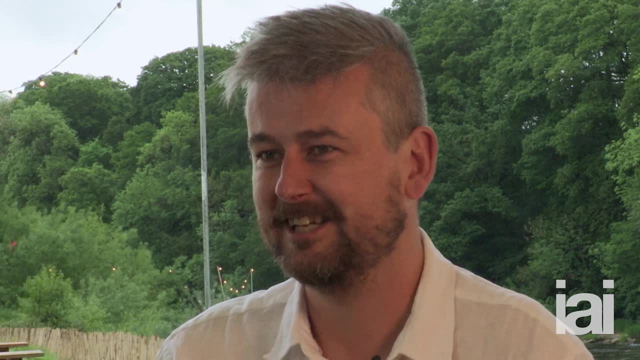 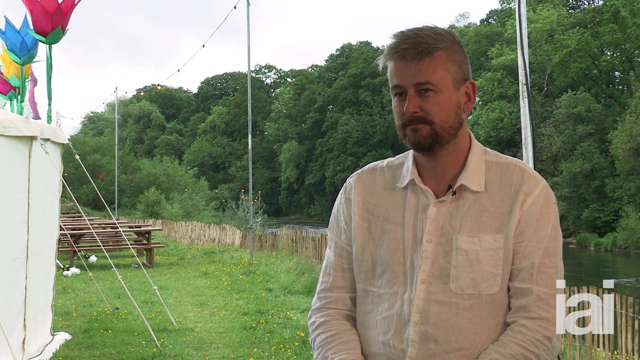 hasn't panned out, So I'm trying a new approach and it's a lot of fun. So this change in starting from the data rather than theory: does this mean that you've sort of given up hope of finding supersymmetrical particles? 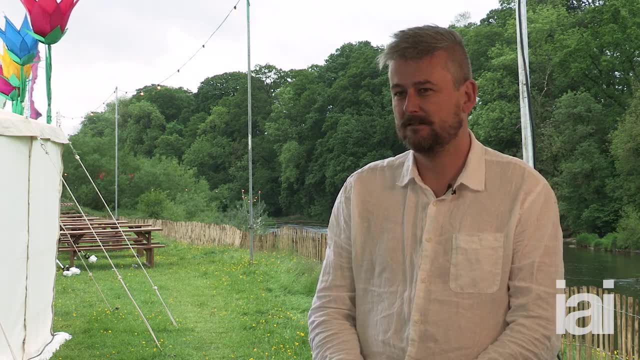 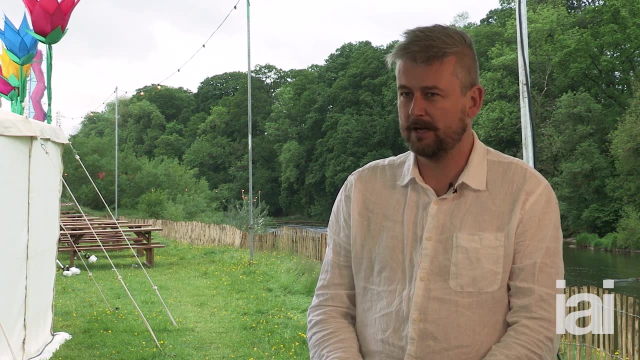 No, Okay. So is the work still focused on that? No, It's focused on supersymmetry. That's just a belief you have, but you've kind of like No, Okay. So looking at my own work at the moment, the way I answer this question is: 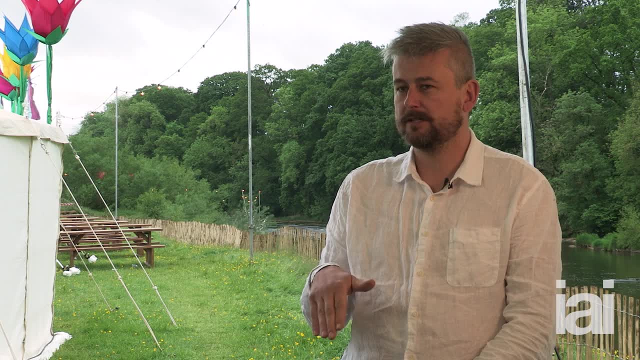 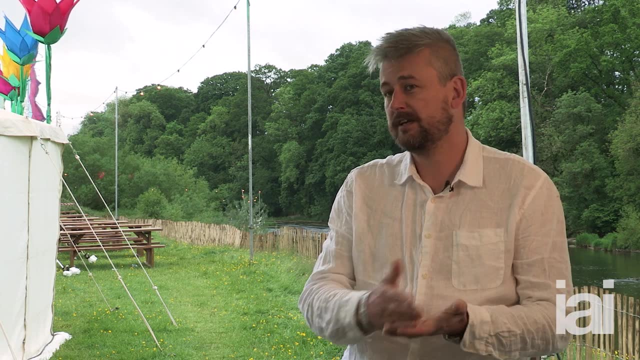 the way for me to make progress right now is not to work on supersymmetry, And the reason is because we know from the data that the Large Hadron Collider has seen already that in the next few years there's not going to be a big discovery of supersymmetric particles. 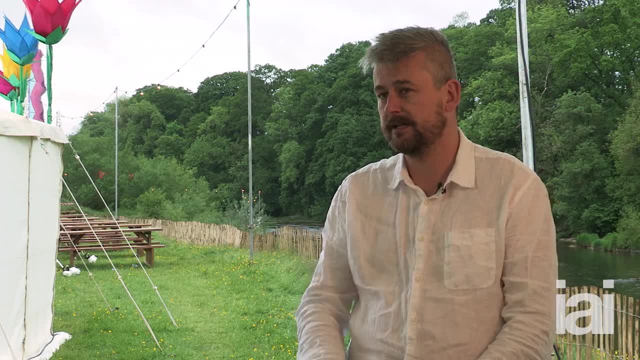 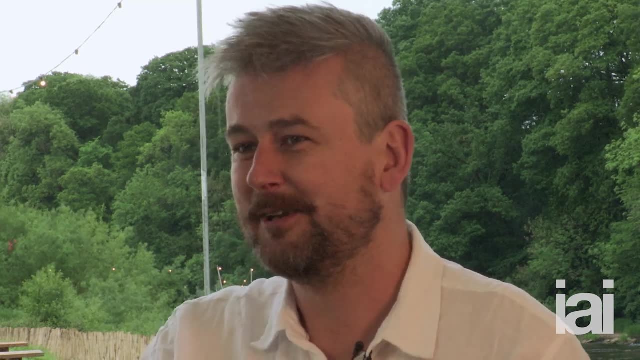 Otherwise we would have seen small, Small fluctuations in the data already. So in the next years, for me that's not where the discovery is going to be, so I'm looking elsewhere. But still, you know you can't help. in your heart of hearts, believe in this beautiful theory which explains a really important 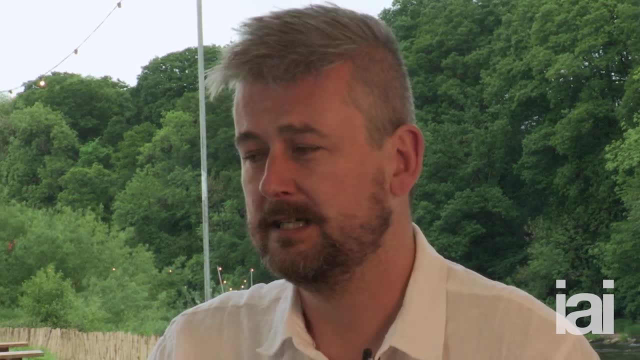 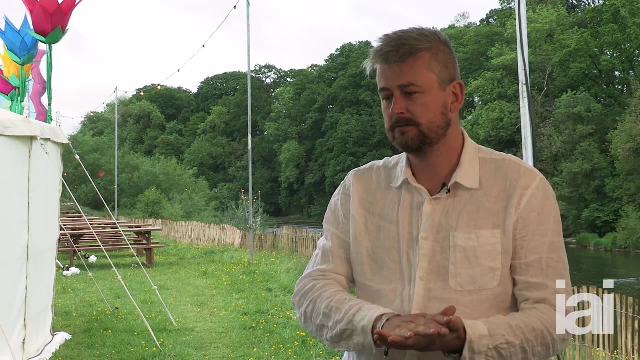 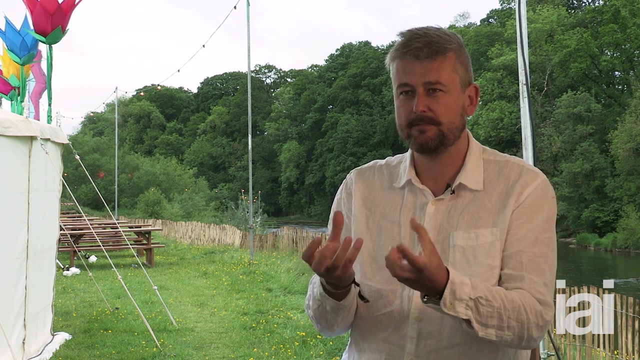 fact that we otherwise don't understand. And that fact is: why is the Higgs boson so light? So if you do calculations on Higgs bosons, they're. They're affected by quantum fluctuations, the seething of space-time in terms of other 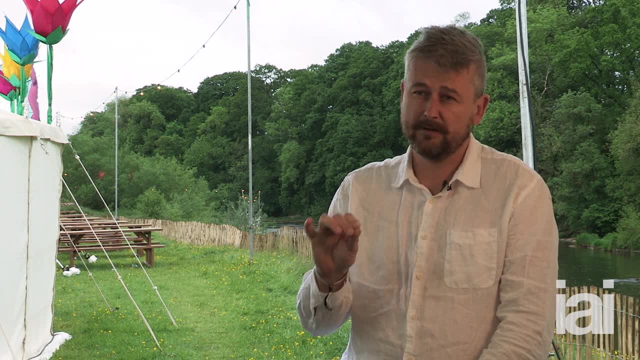 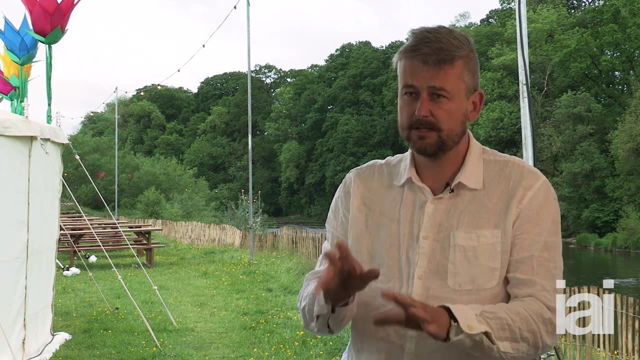 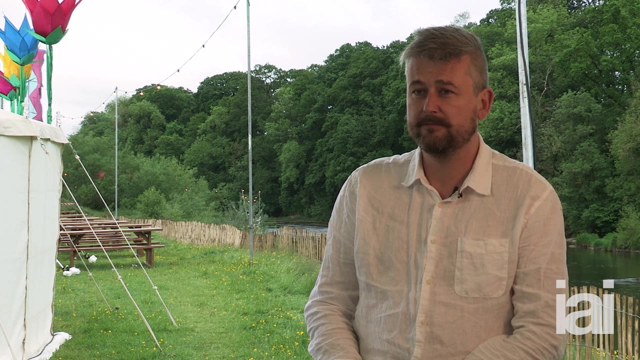 particles, And they're special in that they feel those fluctuations extremely sensitively. And if you do back-of-the-envelope calculations, those fluctuations should increase its mass by something like a billion billion times more than it's been measured to be. So this 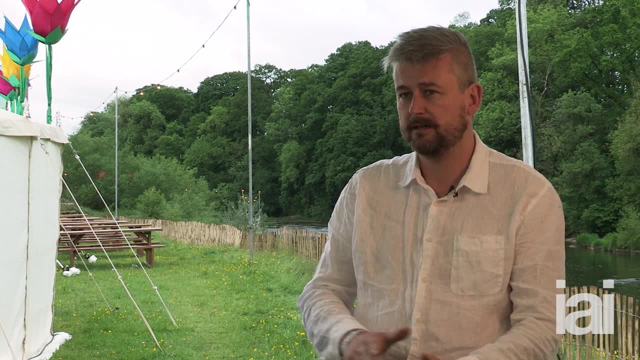 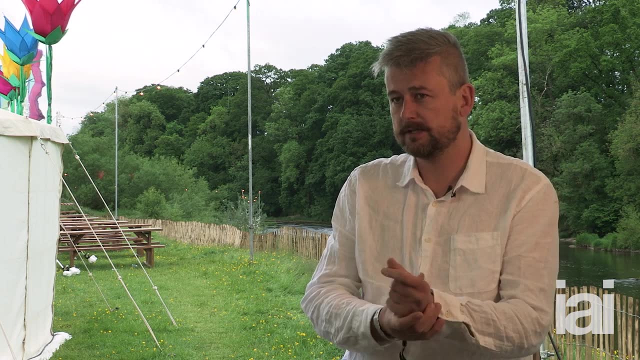 is a puzzle that we don't understand with our current theory. It's not explained why they're so light and how is it able to stay so light with these quantum fluctuations? Supersymmetry explains this. It doesn't mean it's the only. That doesn't mean it's the only explanation. But the other ones don't work or, you know, we haven't really found a decent other one. So that's why we were so keen on it and why we thought we might be able to find supersymmetric particles as a signal that the theory was. 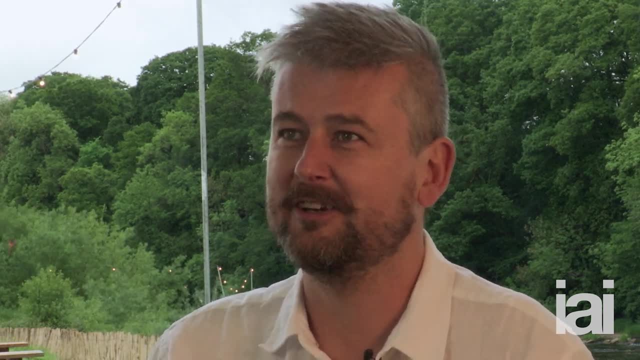 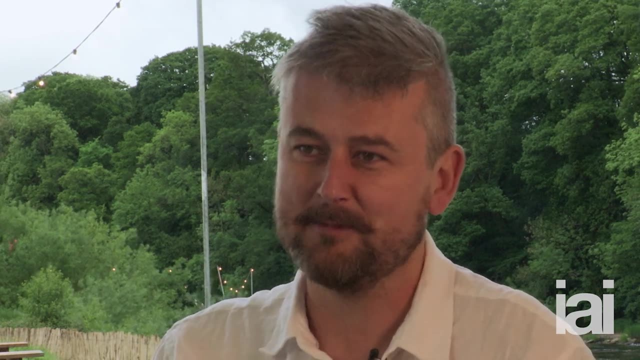 right at the Large Hadron Collider. So you know, if, in I don't know- five or ten years' time, some signals start appearing from the data, of course I'm going to jump right back on it, right? But for the moment, 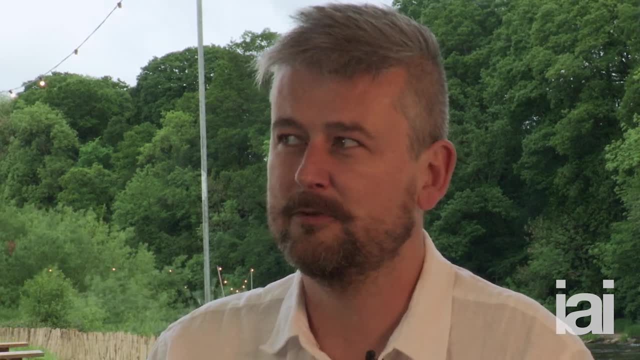 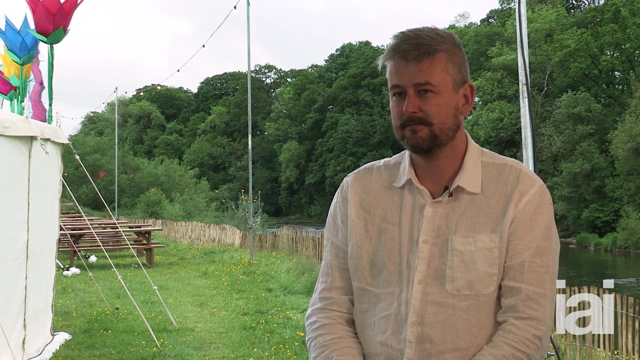 I think, in terms of progress, it's more fruitful for me personally to look elsewhere. And why do you think there is this pull to sort of the grand theory of everything? Why has this been a focus in particle physics rather than starting from the data? 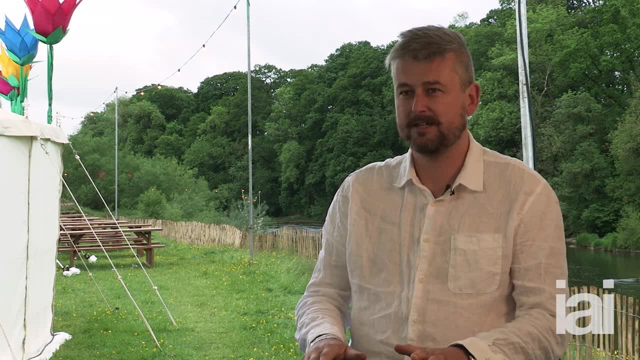 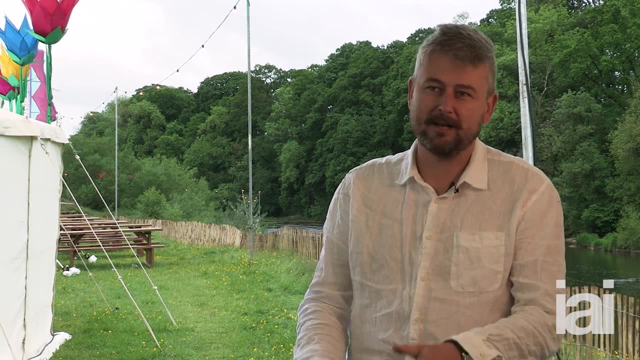 Well, I mean the truth. you know if I'm honest, the truth is that, actually, you know, actually lots of different approaches are taken by everyone, and it's a question of balance, of how much you weight one thing against another, and people work in different ways. 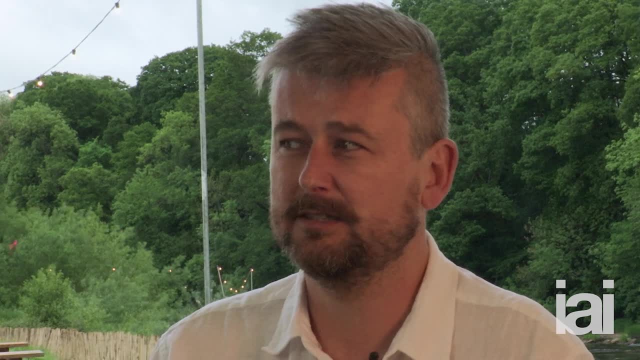 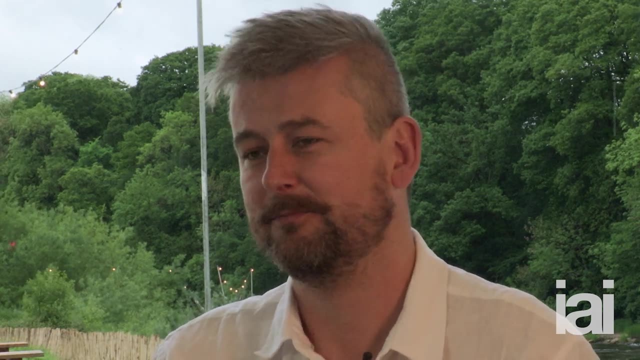 and so on, But the grand unified theories are ambitious. I mean, if you could explain everything in one fell swoop. you know not everything. It's not going to explain how you fall in love, for instance, right, But everything about particle physics and perhaps. 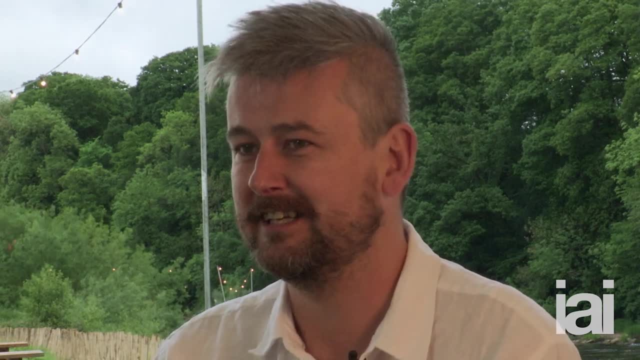 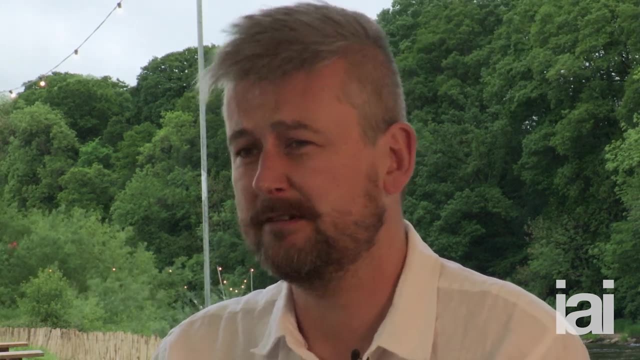 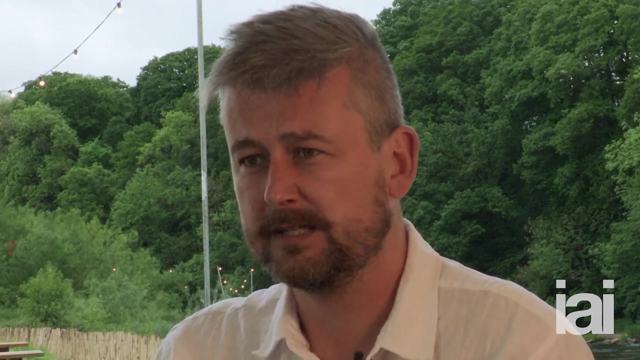 even the early universe. that's a very tempting, seductive idea, right. So that's partly it. But also just theoretical progress was made. I mean, people didn't realize these grand unified theories could exist in the 60s, 1960s. 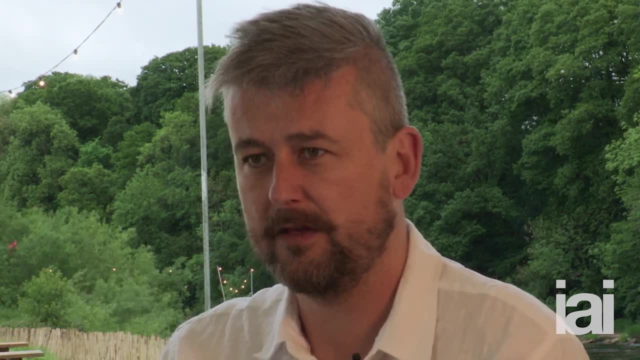 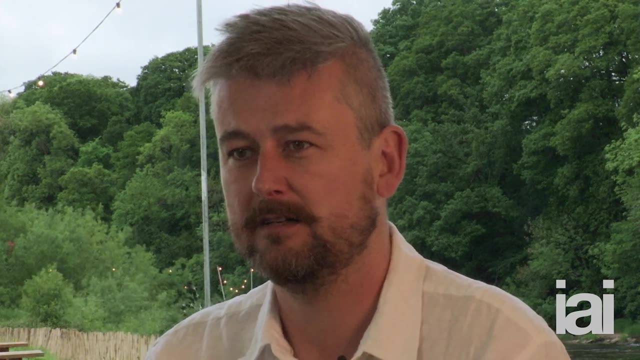 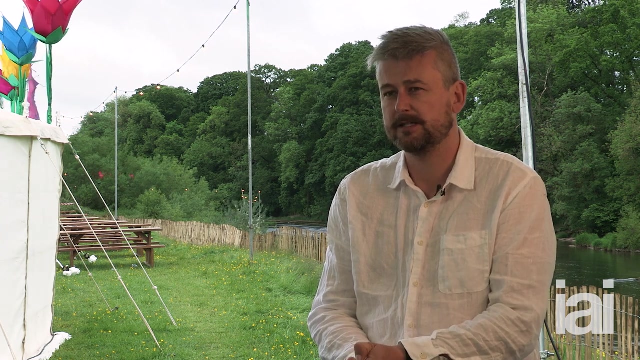 And then later on, you know, they sort of popped out of the theory, And so it was a theoretical playground where potentially you could explain everything all of a sudden, And so there's a lot of activity on it. But they looked for experimental signatures that they would correct, One of the main ones actually. 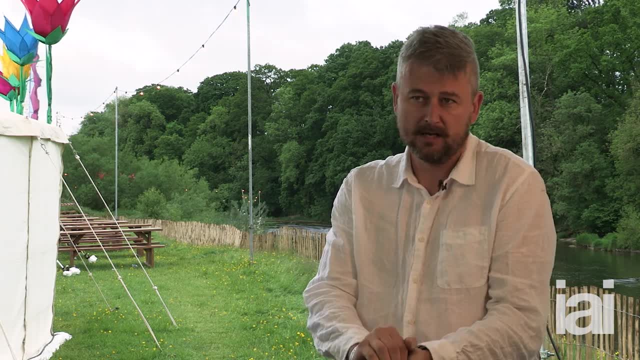 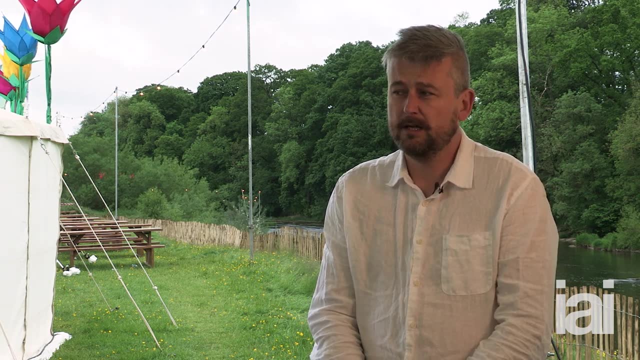 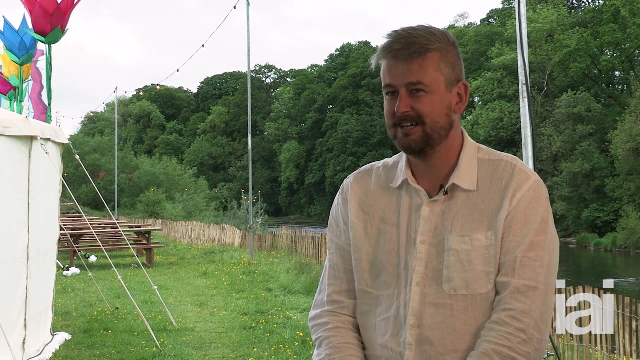 with grand unified theories was that protons, you know the particles inside of atoms, in the nuclear, in the center, they should decay. And they set up this bonkers experiment in a mountain in Japan, in the Kamioka mountain, where they basically hollowed it out and filled. 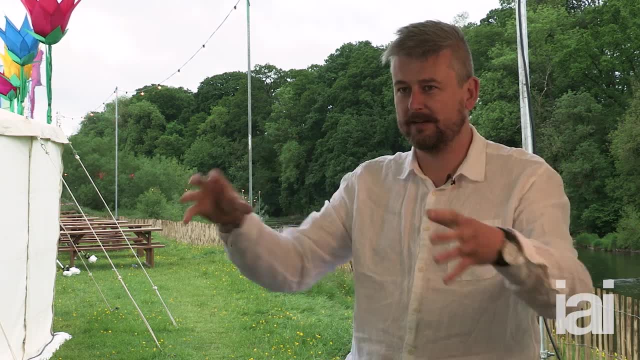 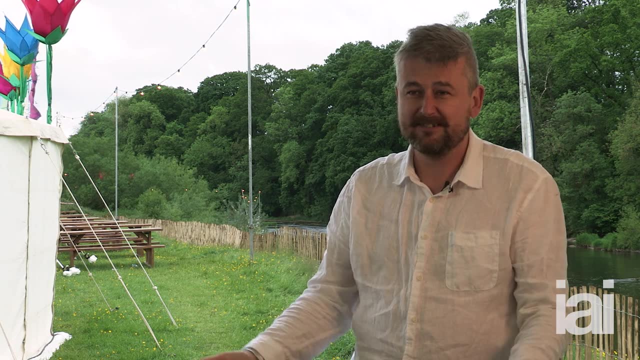 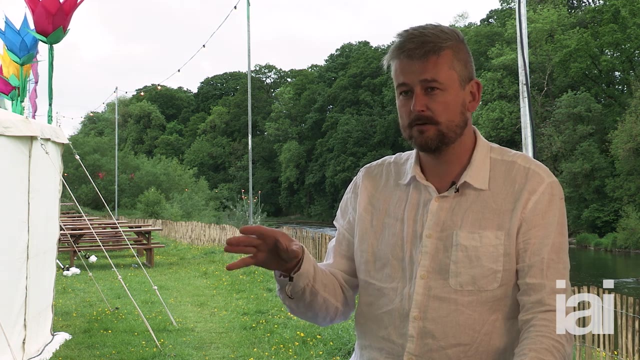 it with water and put all of these detectives, detectors around the outside that measure light, And they looked for protons decaying within the water, basically. So you've got a lot of water, So you know if one of the protons decays you can see it, So you can get very strong bounds on it. on the proton's 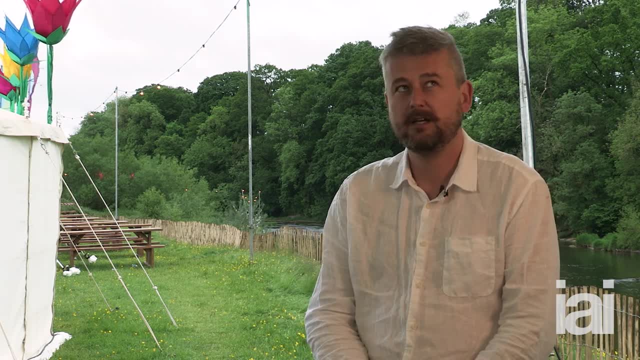 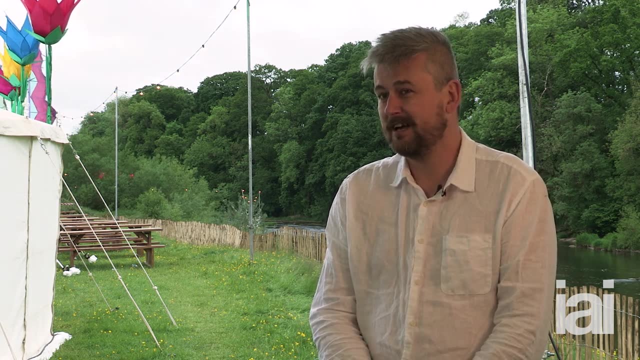 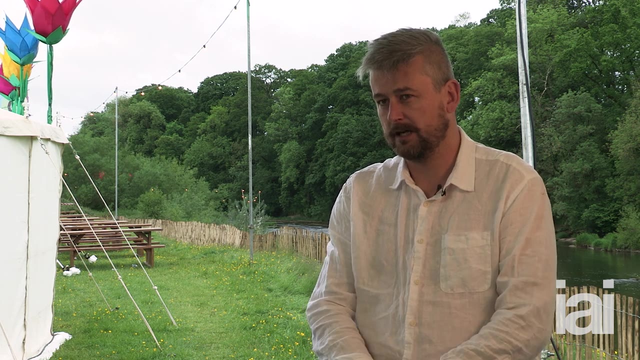 lifetime, because there's so many protons in this water And the current bound on the lifetime is like, roughly it's got to be longer than ten to the thirty-two years. That's much longer than the age of the Union first. So it's challenging the grand unified theories and pushing them, And when you don't, 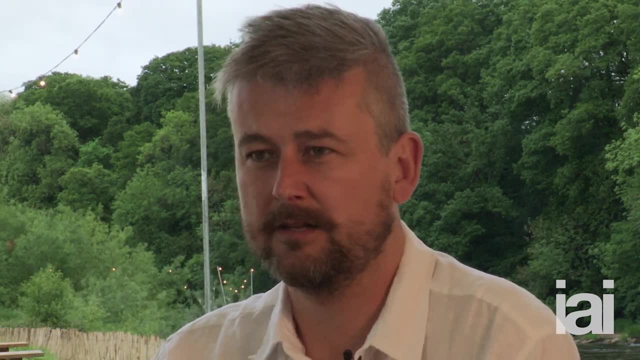 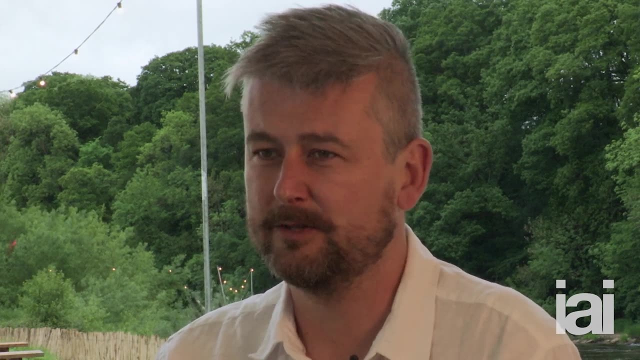 have a good experimental signal that the theory is right. I mean, you don't know where to go with it. You can do lots of theoretical work but in the end you don't really know whether your theory is right or not. And you've written that particle physics is in crisis. Is it to do with this focus on? 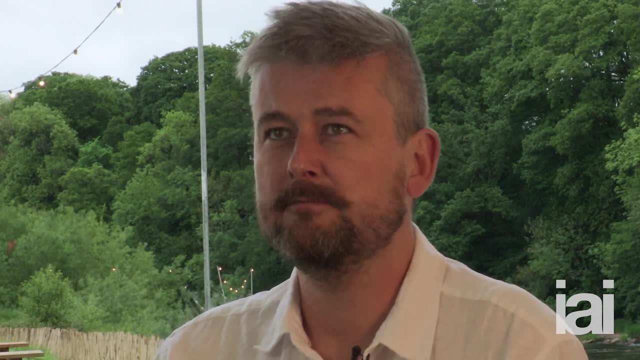 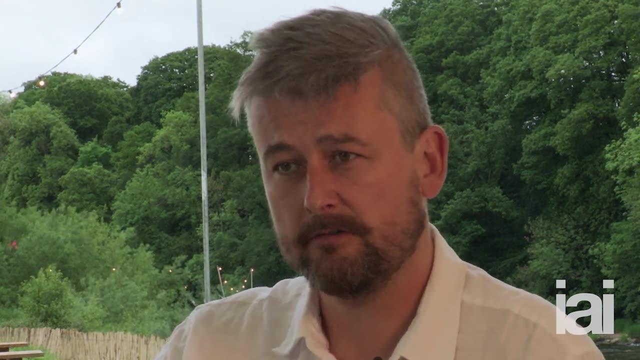 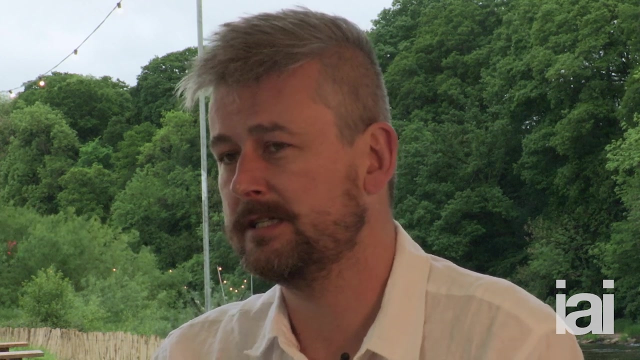 theory. So I don't really. I don't think that's the big crisis. I think there's a crisis in terms of the Higgs boson and this hierarchy problem And the fact that supersymmetry doesn't seem to be right and we don't understand why the Higgs boson is so light, I think in theoretical. 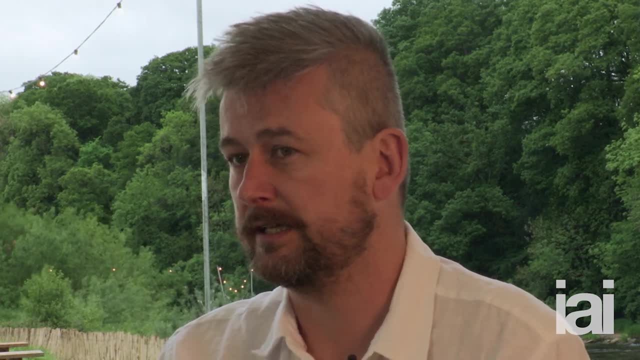 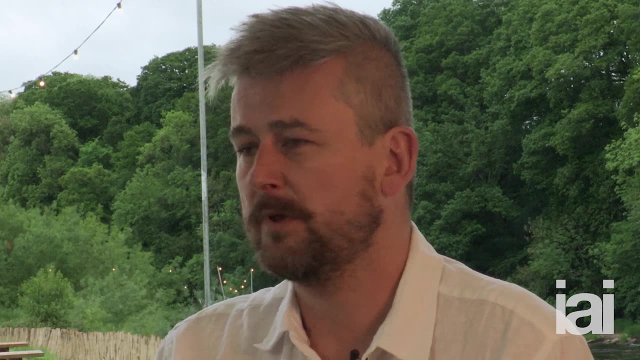 particle physics has a problem with that and we don't understand it, And it may mean that we need to somehow shift paradigm. Maybe there's something going on. Yeah, I think it may be that with the Higgs mechanism, the mechanism by which all the particles get, 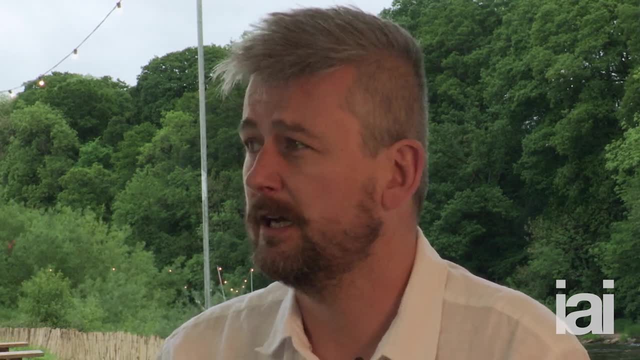 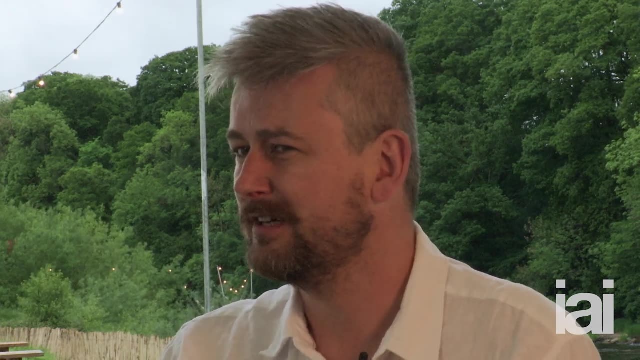 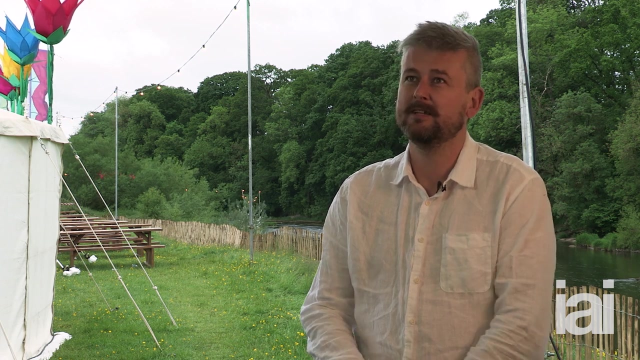 their mass. subatomic particles get their mass. Yeah, So it may just be that there's a puzzle. We need a shift of perspective to really understand that. But yeah, It may just be that. But I don't think that the whole subject is in crisis because we've been too theoretically. 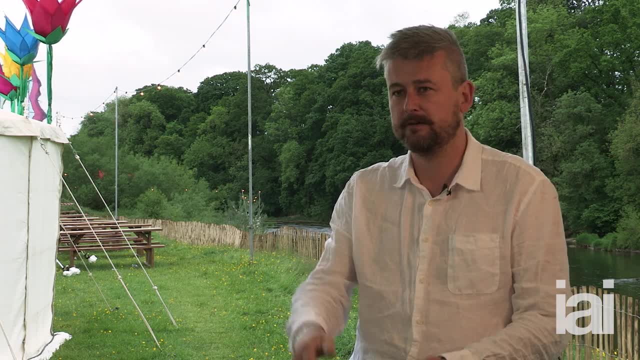 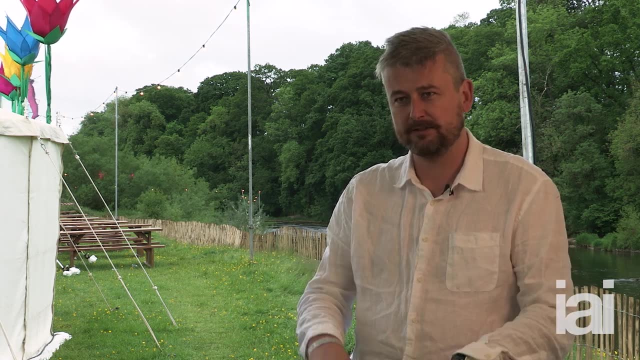 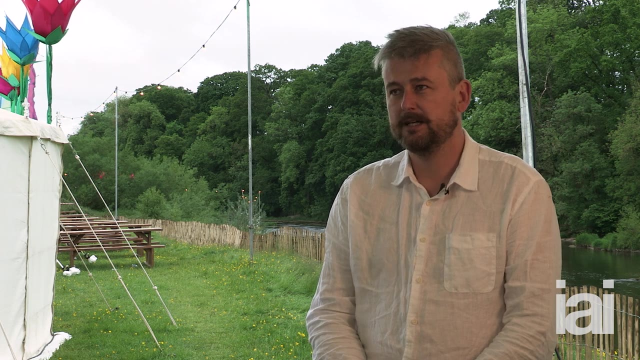 driven experiments are going on and there are people who work in various ways. within that Last century- actually, it was mainly well- we had Einstein and Dirac. they were the big top-down theoretical physicists, you know, inventing things from pure thought and mathematics. 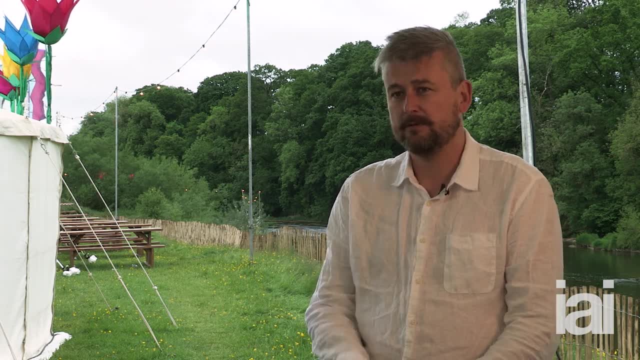 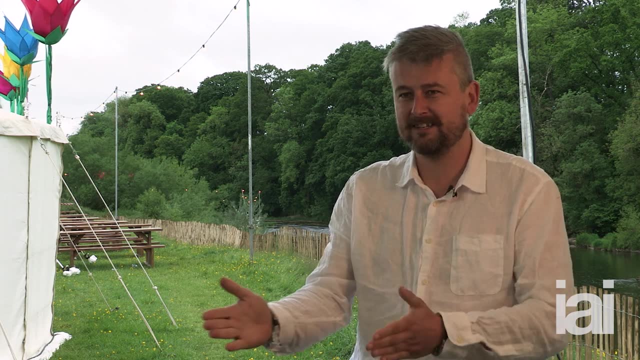 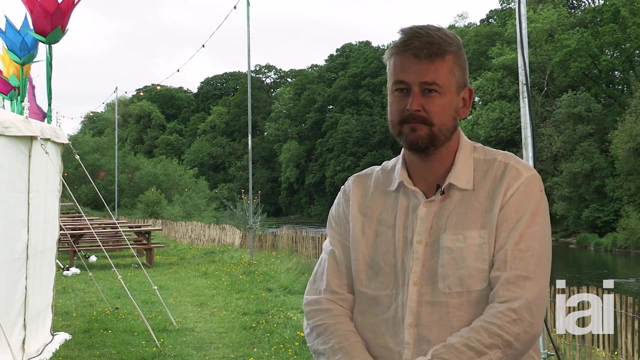 And they had some very big, impressive successes with that. But most of the other progress from my point of view in particle physics was either bottom-up or it came more from a batting back and forwards, an interplay between theory and data, And so all of that continues at the same time. 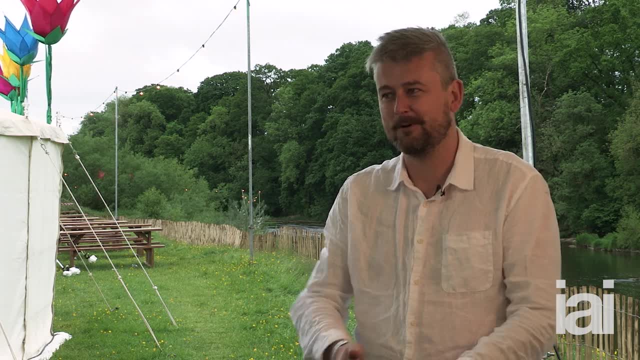 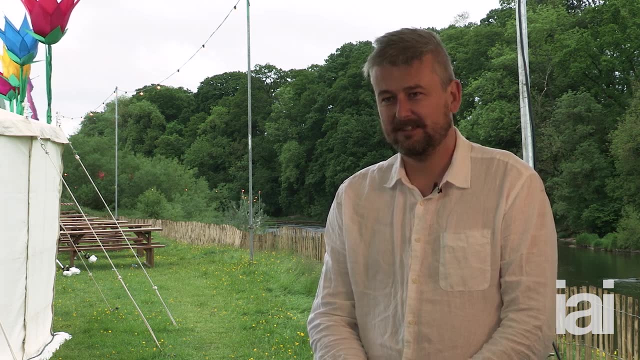 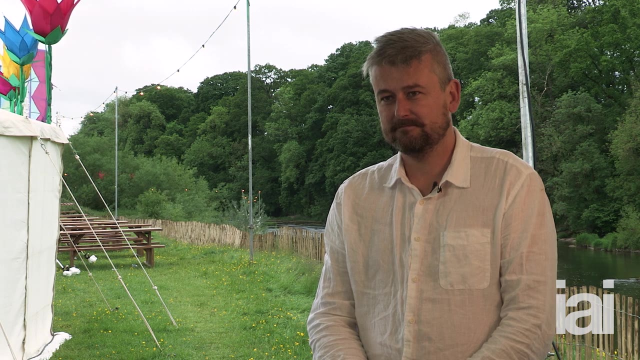 It's more that I've just changed the way I'm working and hope to make more progress. this new way, yeah, And are there equivalent big names of physicists who use sort of bottom-up process that you've been inspired by in your own work, like comparable to Einstein, who is famous for top-down theory? 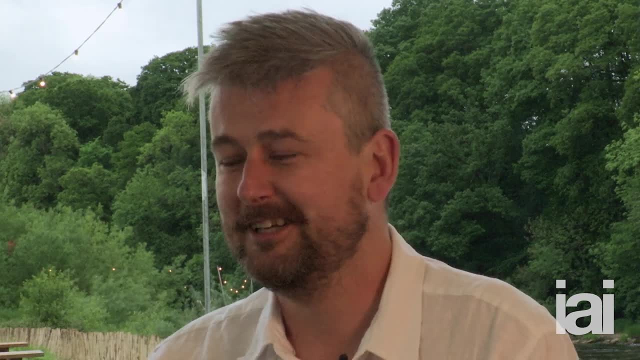 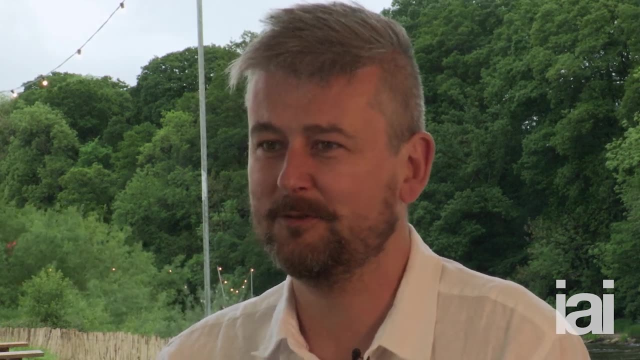 I think the top-down, The top-down theorists I mean they're very clever people. They get more of the big names, but there are certainly some good. You might call them phenomenologists, people who work bottom-up- Bill Cain, for instance. 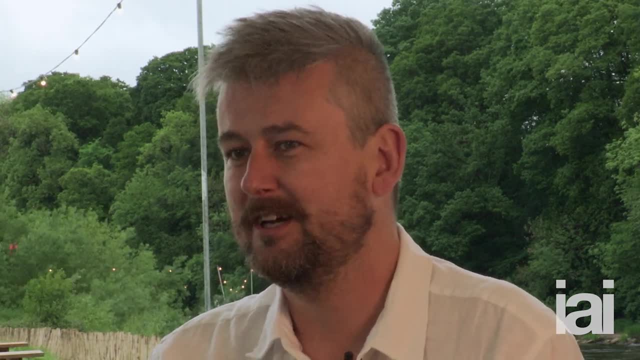 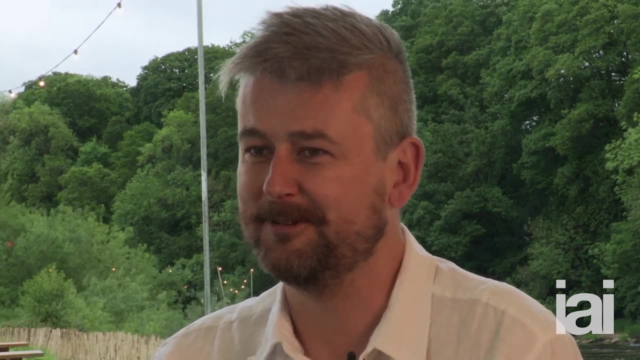 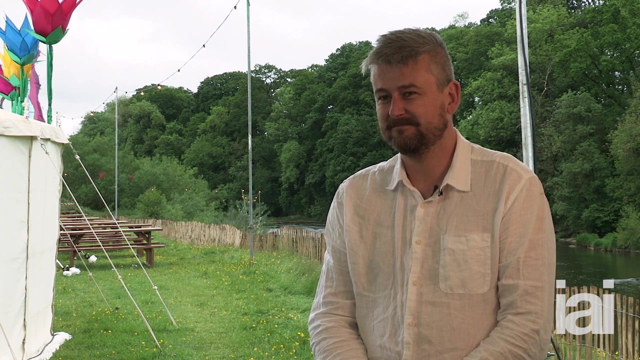 and some other physicists you probably won't have heard of as much, And some of the top-down people also did bottom-up. I mean, if you're sensible, you use everything you know available to you. I guess, Yeah, And the work you're doing at CERN, like in regards to the Higgs boson? what sort of data? 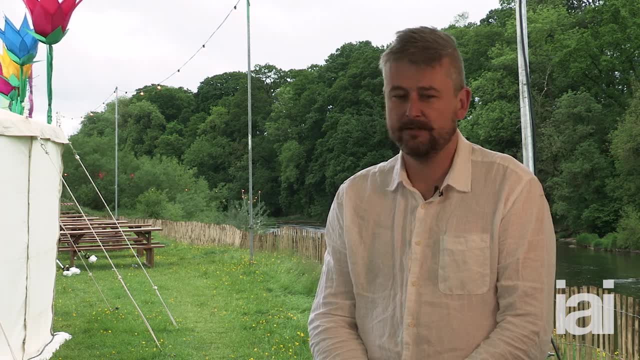 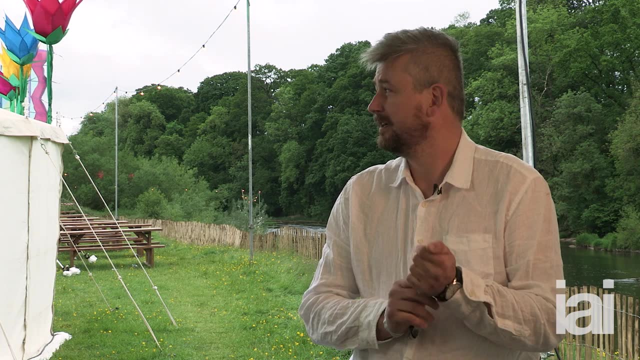 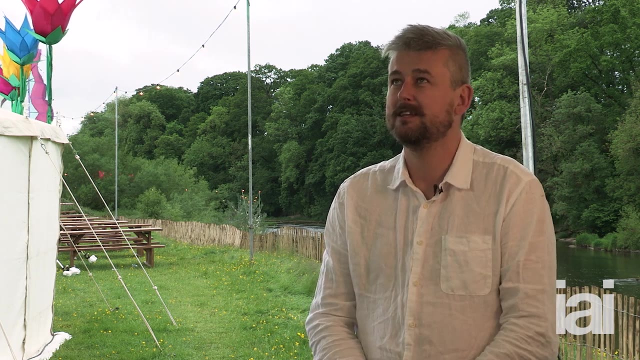 are you using there in more detail? Yeah, So at CERN, protons are collided at extremely high energies. It's 14,000 billion electron volts worth of energy in the beam. well, 13,, actually 13,000. 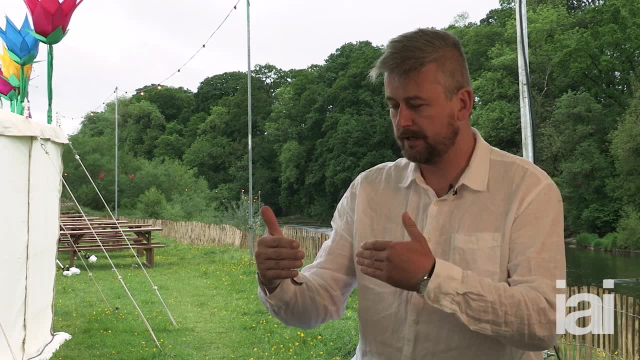 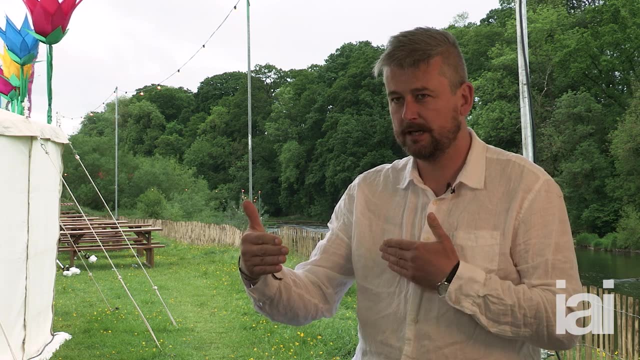 And so, Yeah, So what you do is you put a detector around the point where you cross the counter-rotating beams, So these act like 3D cameras, And what comes out is a spray of 1,000 fiery fragments. 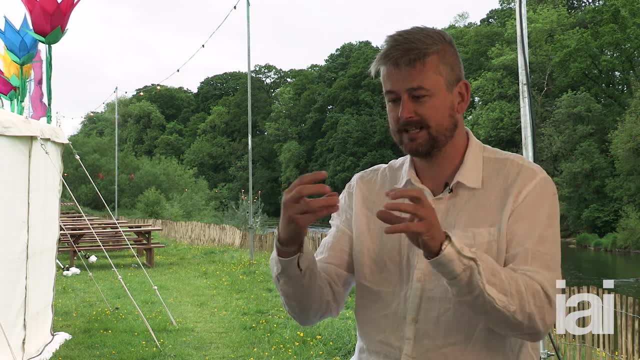 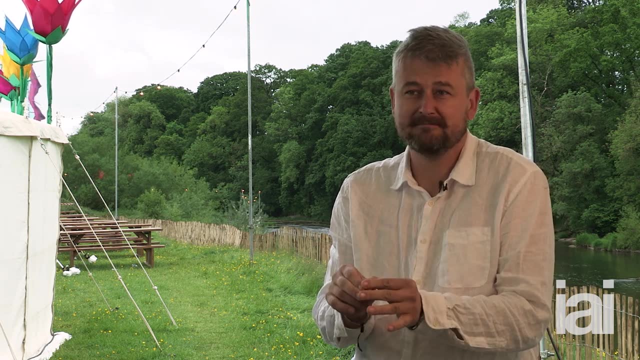 And so what you're doing is detective work: to kind of go back in time, look at each collision and try and work out what was going on right at the center and which particles existed for a fleeting you know fraction of a second. So that's how the Higgs boson was discovered, actually. 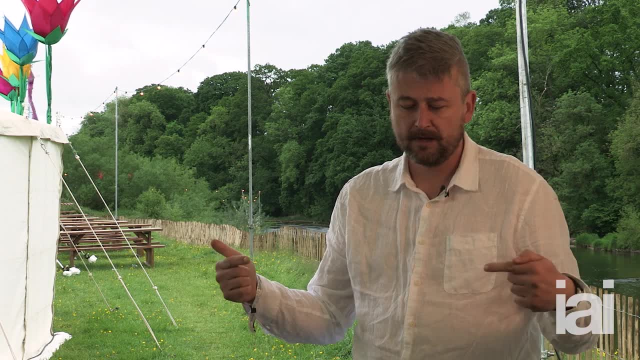 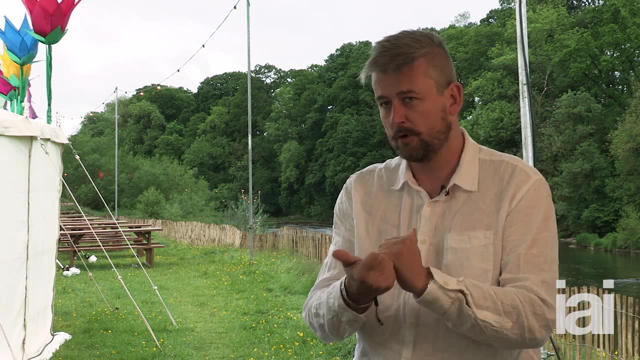 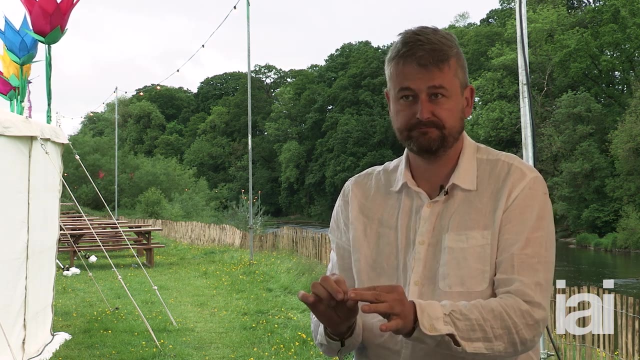 The discovery channel was when they decayed into two particles of highly energetic light. So you get two photons going more or less back-to-back with particular energy. So their energies add up to the mass of the Higgs boson. okay, So through Einstein's equation, E equals MC squared, you're turning the energy of the beams into the mass of the Higgs boson, which then goes into the energy of the light. So that's So you do various bits of detective work. So the Higgs, a particle which is very much like the standard model Higgs boson, was discovered. 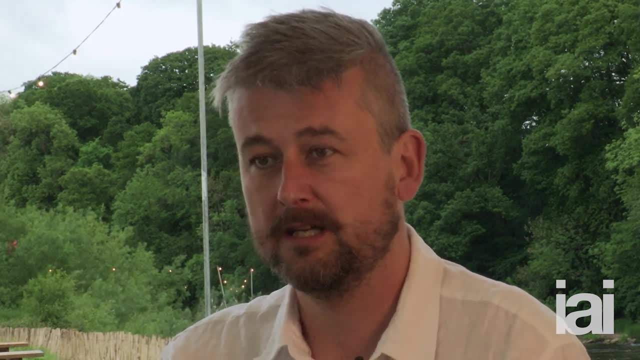 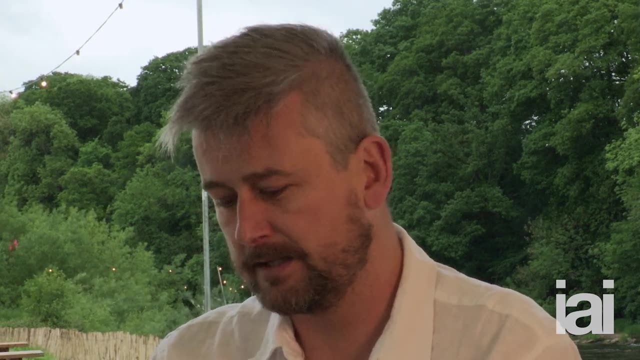 But then you want to check. you know, does it behave in all the different ways like it's supposed to Have? we really got a hold of the theory, So it's As well as going into two particles of light. the chance of that is like 1 in 500.. It just happens that it's easy to spot those ones, But it also decays in other ways. So you check to see if the frequencies all agree with the theory, And so far they pretty much look like the standard model has got it bang on. 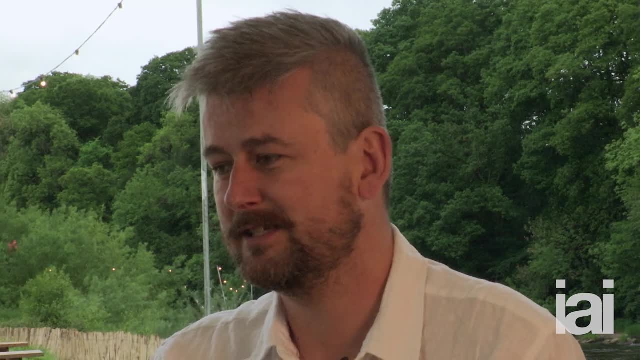 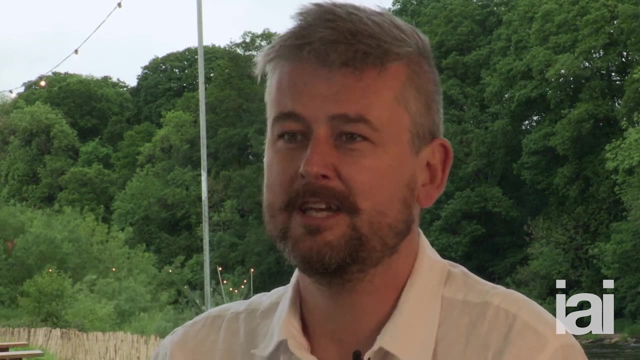 So we've got this dichotomy where the standard model is telling us that the experimental signatures of the Higgs boson all agree with its predictions, But then we use the theory to try and estimate the mass of the Higgs boson and you get it. 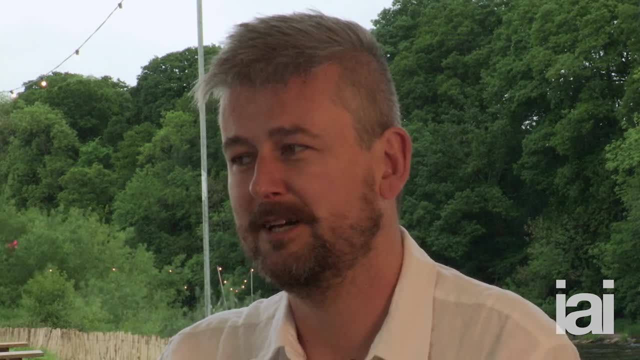 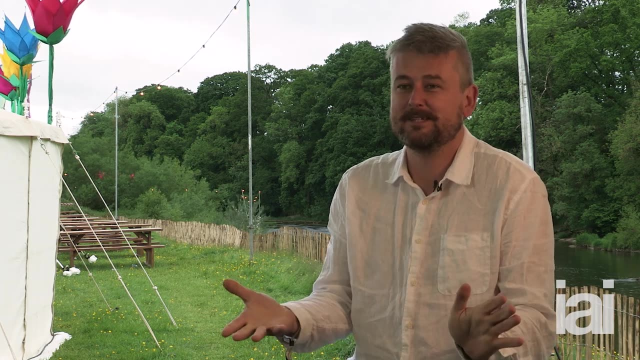 right by Wrong, by some huge factor. So it's an interesting thing, Okay, It's an interesting situation to be in. Yeah, And that was the thing. If we had supersymmetry then we'd understand it all, But we don't. 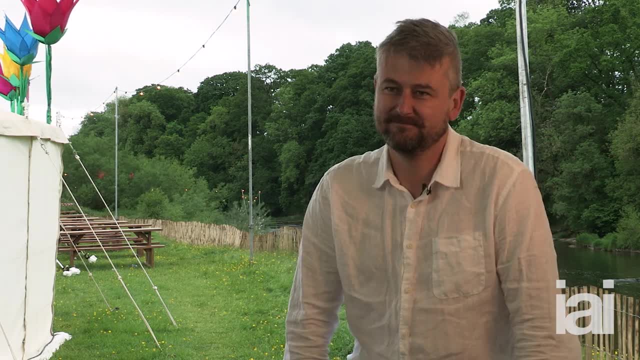 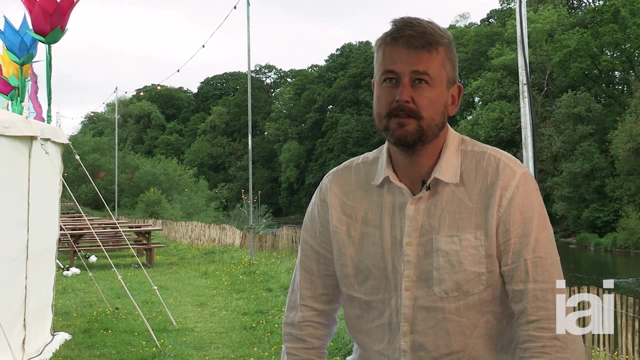 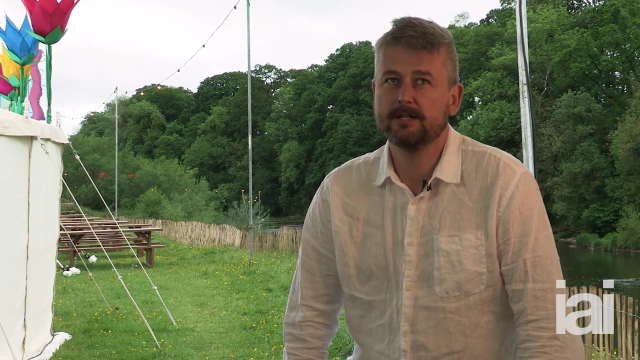 And what would the ramifications be of understanding why the Higgs boson is so light? Why is that sort of a barrier at the moment in theoretical physics? Well, the big, I mean. we want to understand how particles act. We have this. 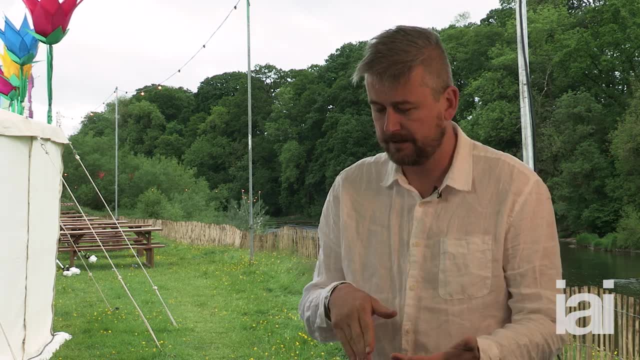 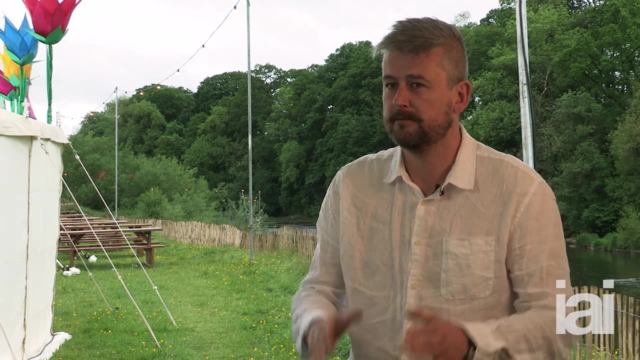 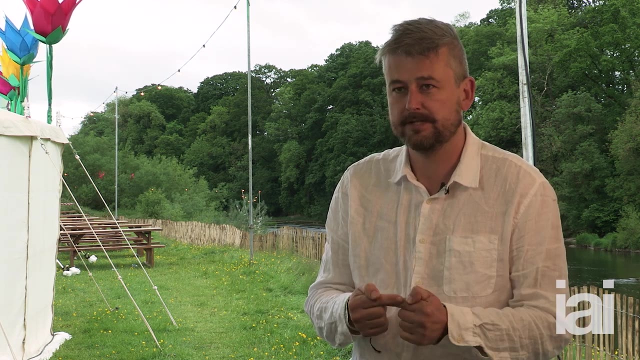 Yeah, I mean particle physics is a list of all the particles that have been discovered experimentally, including the forces, But it's a mathematical quantum field theory. It's a mathematical framework that tells you how they act. It can predict precisely for you what the frequencies of various things happening are. 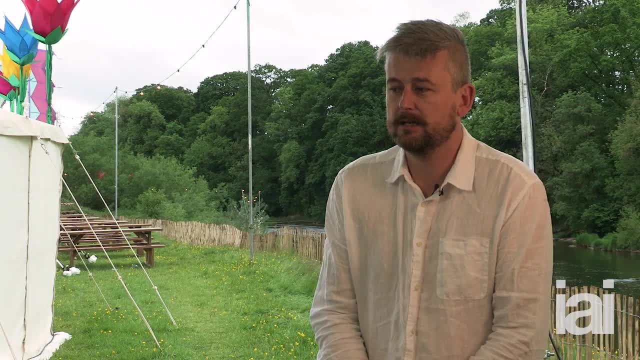 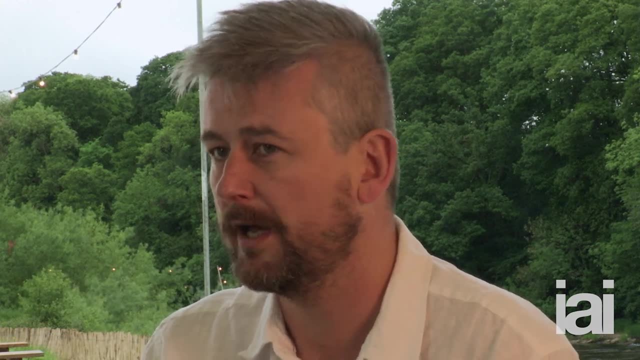 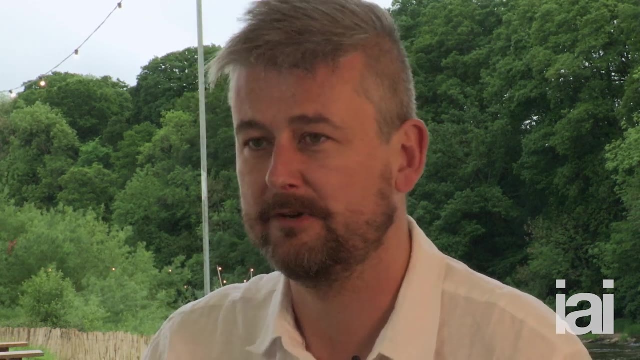 when you do these collisions And if you just use that theory, it's successful in nearly all ways. Yeah, It's one way of predicting the Higgs mass. So it's like a chink in the armor of this whole machinery. And, of course, chinks in the armor if you can find out why it's gone wrong, then you 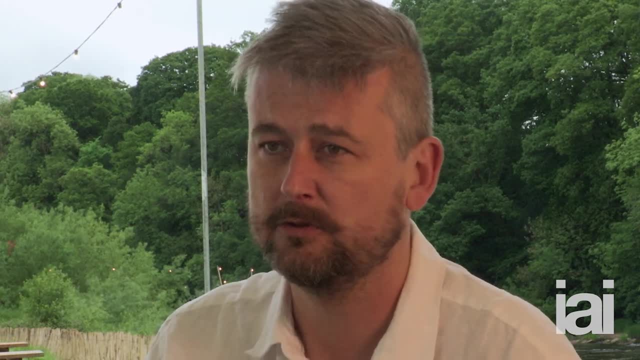 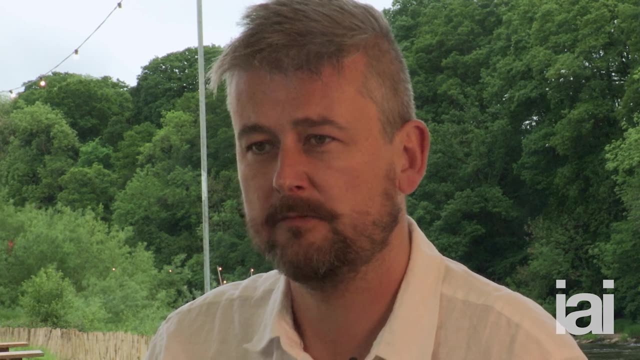 go through to the next stage. you make a big discovery and we just find out more about the universe. So this is pure blue skies research. We just want to find out about the universe and the way it works. It's not particularly application driven. 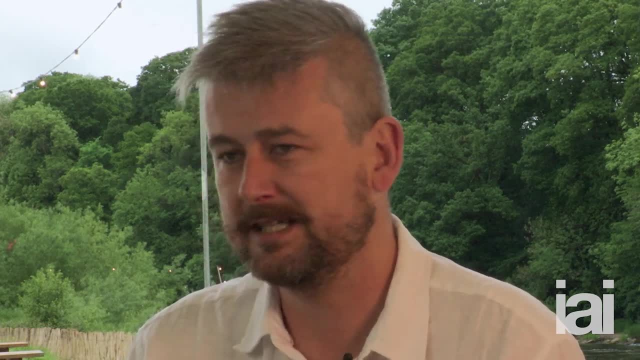 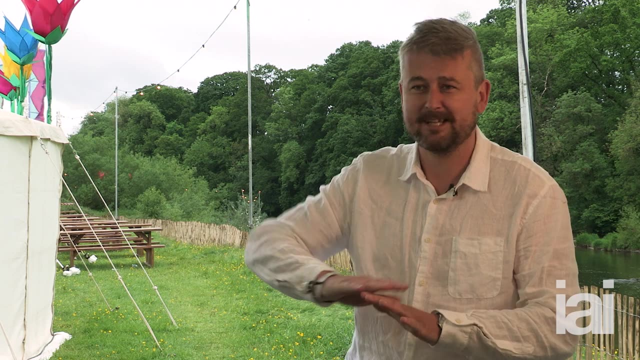 You know We're thinking a lot of turning mass into energy and vice versa. So there may be some hopes in the future for energy generation, But this is like way off. I mean, at the moment we're just trying to find what's going on. 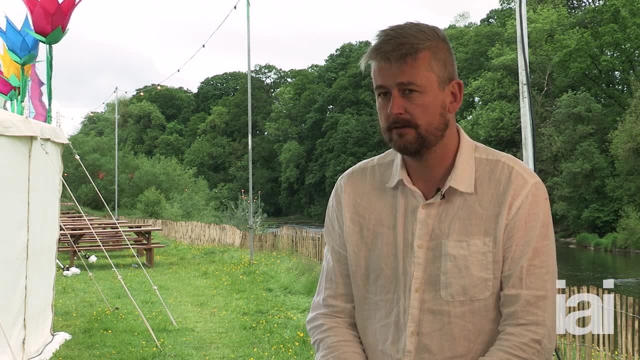 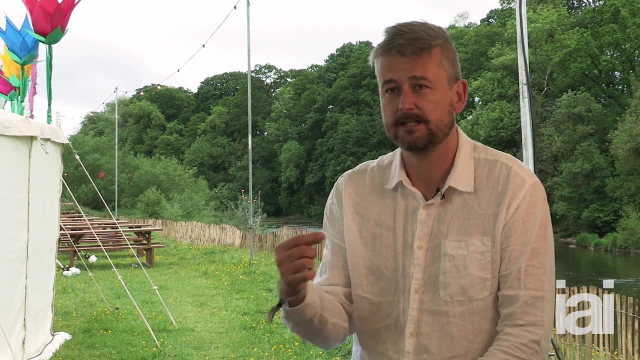 There's also work on proton therapy going on And it's basically accelerating protons using much, you know, very similar techniques that they use at CERN, And so there's R&D going on to that And it can be good for various deep kinds of tubes. 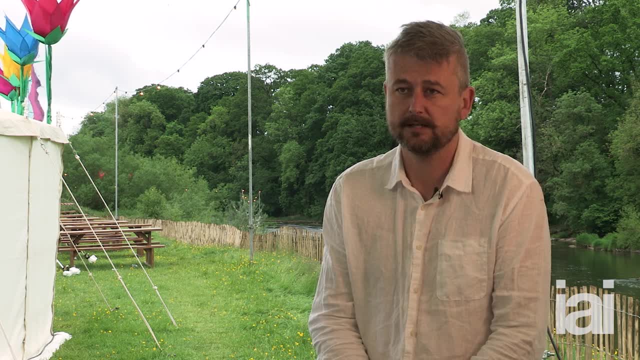 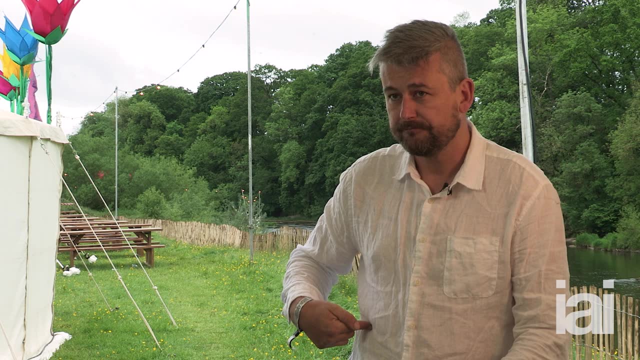 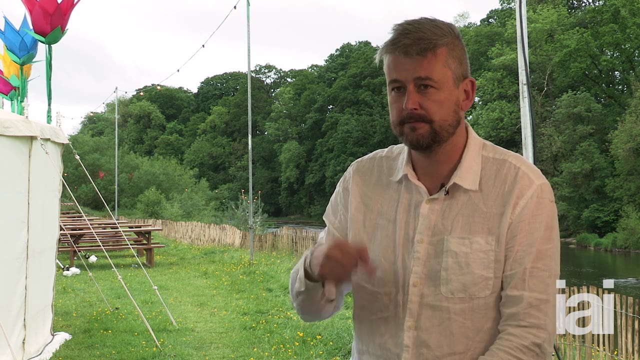 Yeah, And there's a lot of tumors and so on. for treating those things. How does that work? Well, you basically fire the proton beam into the body And it dumps all the energy at a certain depth. So when you've got very deep tumors it can be very damaging to the tumor, but not so. damaging on the outside. So for certain kinds of cancer it's indicated, whereas other treatments, you know it might damage the rest of the body too much, So it can be more localized. So in certain cases it's very useful. 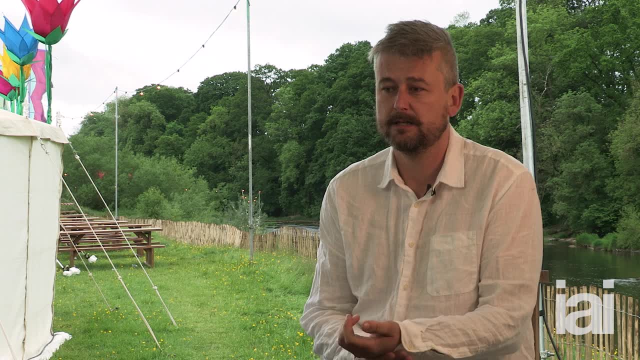 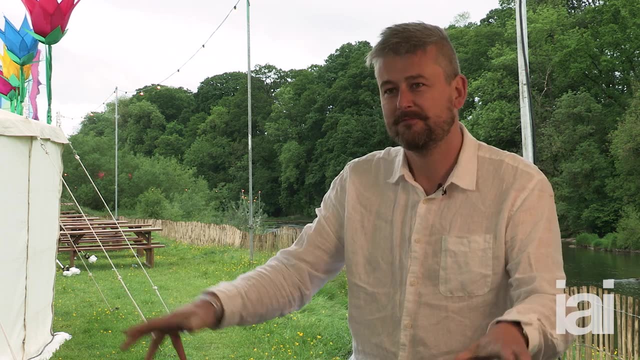 And there are proton therapy treatment centers. There's now one in the UK and there's another one being built. I think Yeah. So it has all these spinoffs, you know, because you're pushing technology further than it's been before. 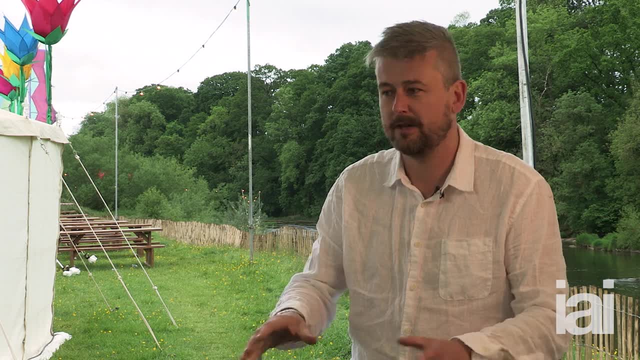 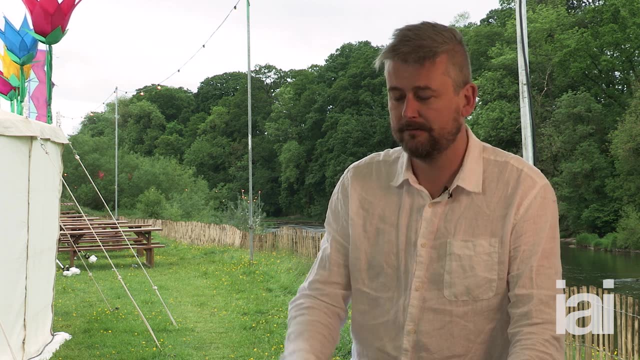 And of course there are uses for it, And so CERN's engaging with medical physics and all sorts of things. So, for example, cancer, Yeah, And CAT scans- If you get CAT scans these days, the modern version of that was invented by the medical 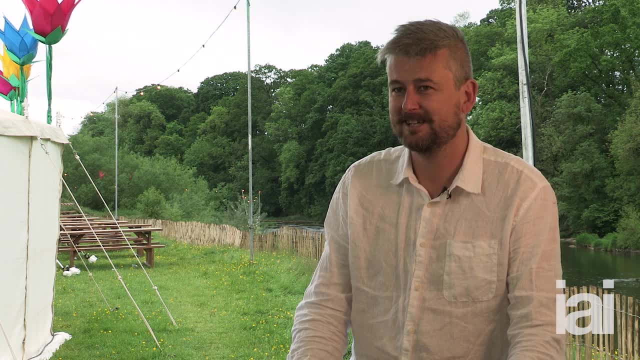 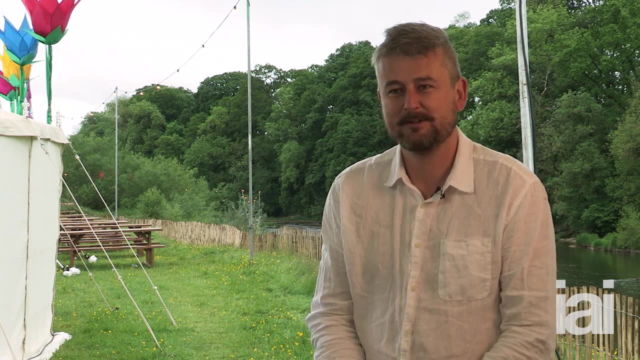 physics team in CERN where it takes x-rays and, you know, builds up a 3D picture at the same time. So, yeah, there's all sorts of good stuff kind of coming out of it that's directly relevant to society. 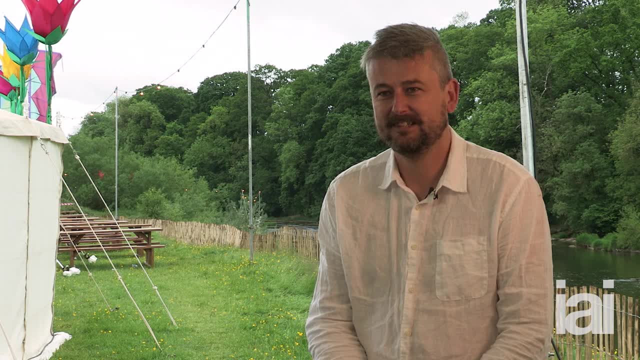 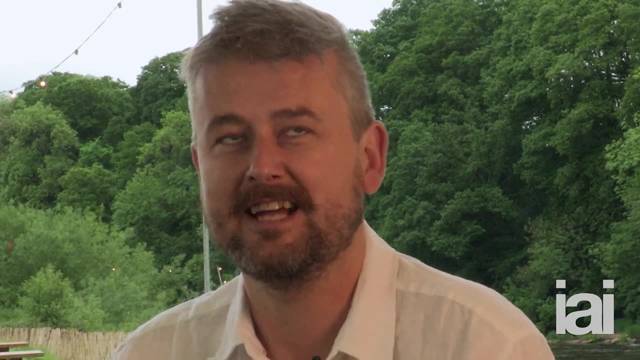 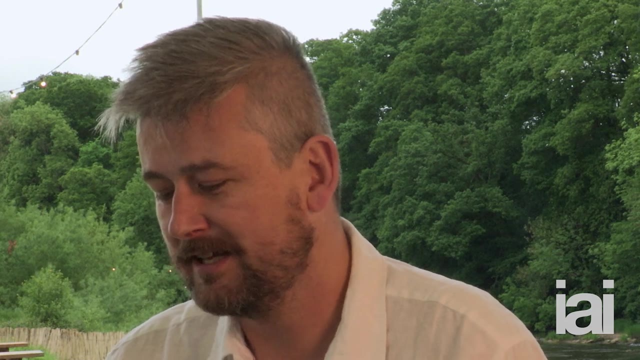 And are you hopeful that you'll work out why the Higgs boson is so light? Yeah, always hopeful, Never give up. Yeah, I've got no good ideas at the moment, but we will see. At the moment, actually, I'm looking at other data. 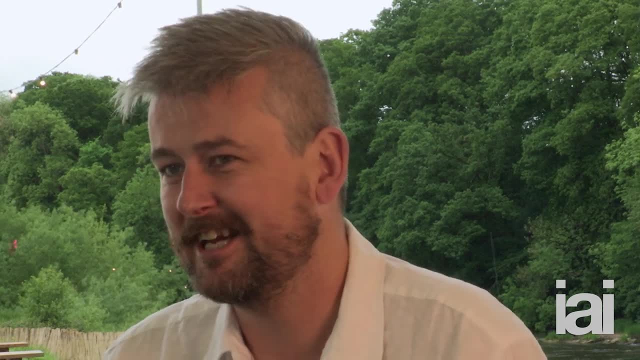 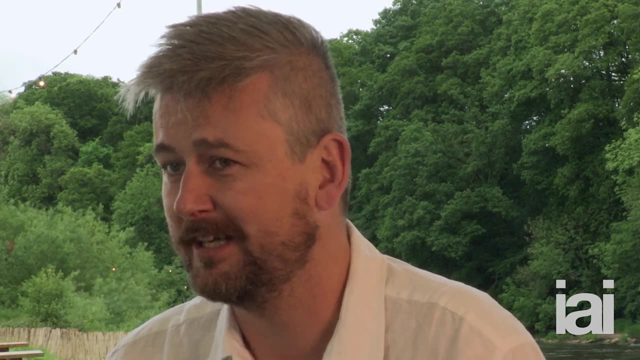 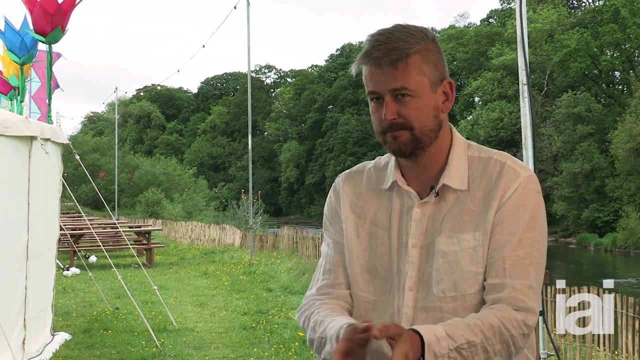 There are these particles called bottom mesons and they're decaying with the wrong frequencies. So I think there's a glitch in the data. So that's an opportunity for me. So we think there might be a new force which is breaking up these bottom mesons. 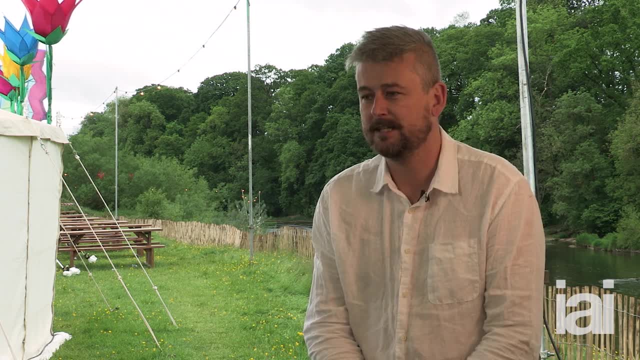 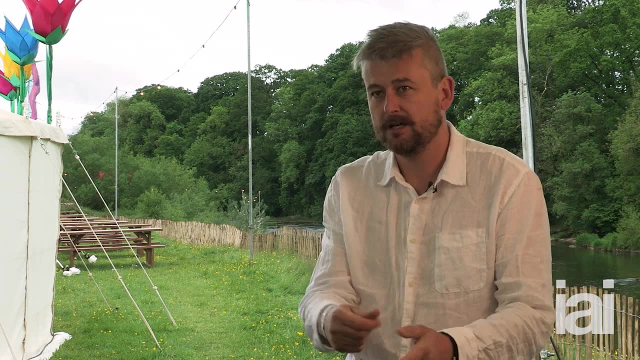 These bottom mesons with the wrong frequencies, And so, yeah, we're proposing ways of testing that theory at the moment. So this is this bottom-up way of working. just found a glitch, proposed something which doesn't necessarily explain anything else, but just to explain this data. 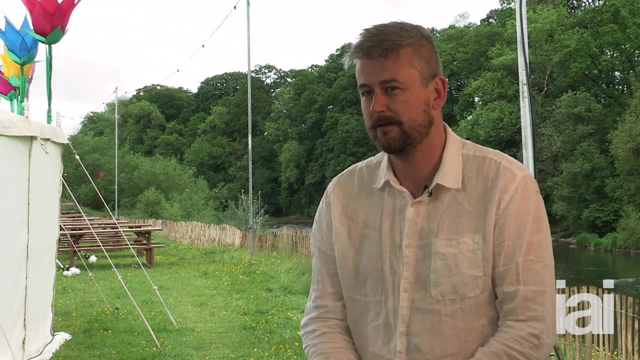 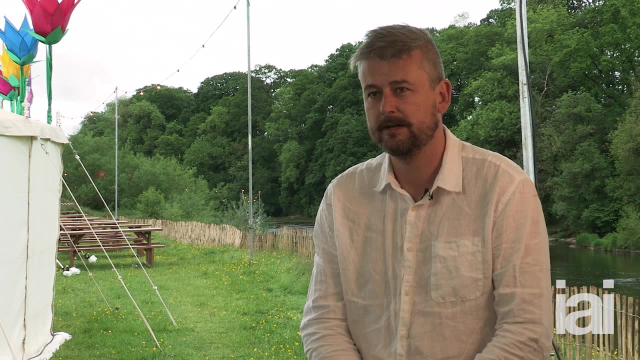 But then now we're starting to ask: well, what does that mean? You know, if there really is this new force, what else can it explain? And so we're starting to build a theoretical framework around it. It's a lot of fun.